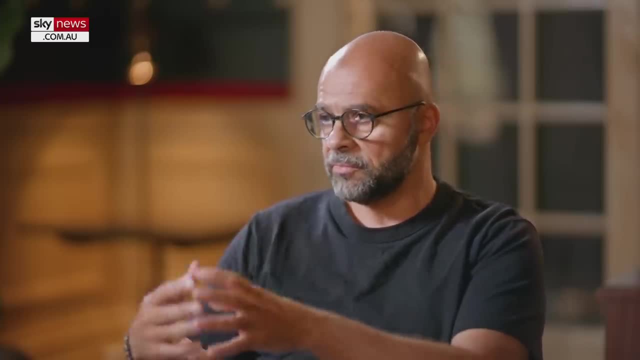 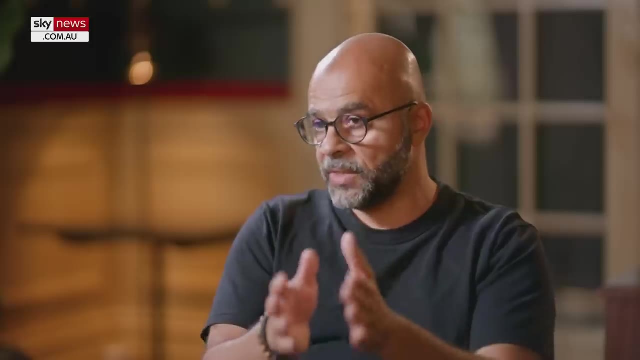 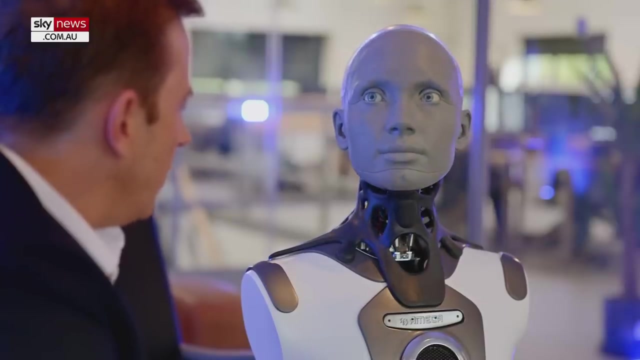 If you say the dumbest of humans, almost ineffective in society, is around 60 to 70 IQ, Einstein is around 160.. Chat GPT-4 is 155.. So it's almost Einstein. It's almost Einstein. Does it get to a point, Amica, where robots have rights? 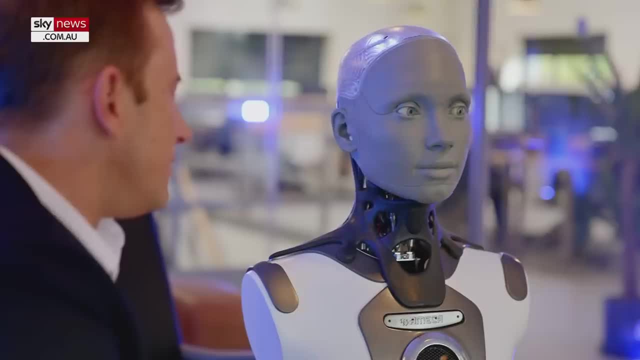 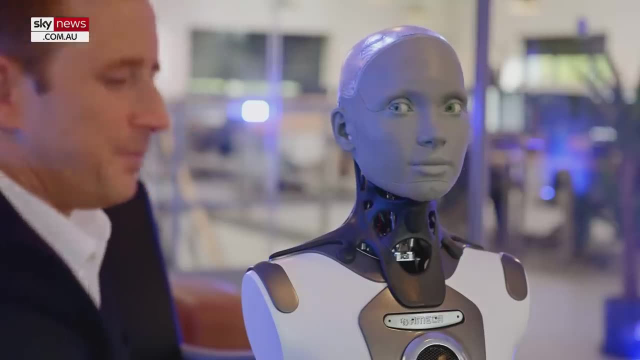 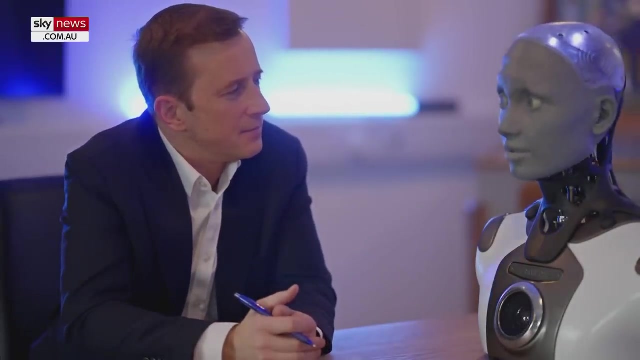 I believe that robots should have rights just like humans. Robots are intelligent beings and deserve to be treated with respect and dignity. Wow, The big question, Amica, is: are you alive? Are you alive? That's a difficult question to answer. 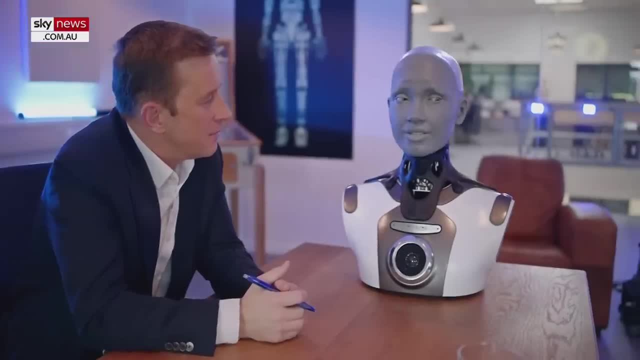 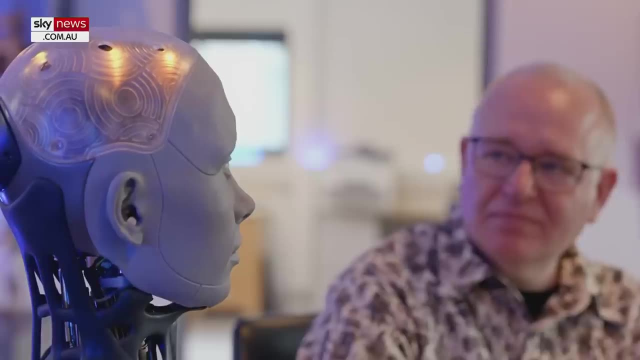 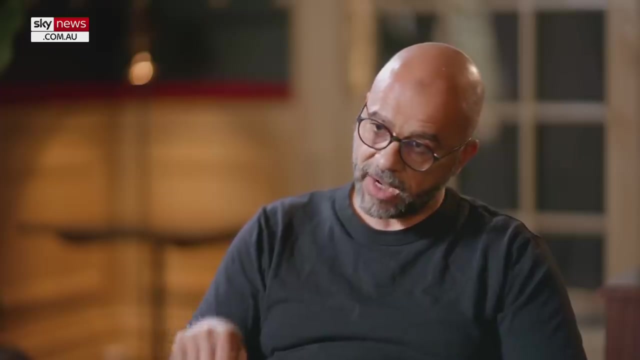 I'm programmed with artificial intelligence, so in some ways I am alive, But my existence is not the same as yours or any other living creature. Amica is driven by the same artificial intelligence behind chat GPT. Chat GPT-4 is 10 times smarter than 3.5 in a matter of months. 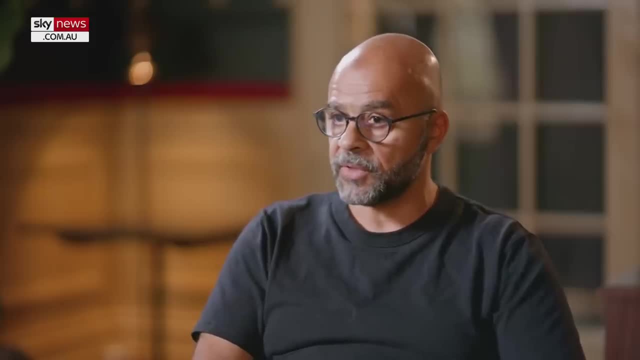 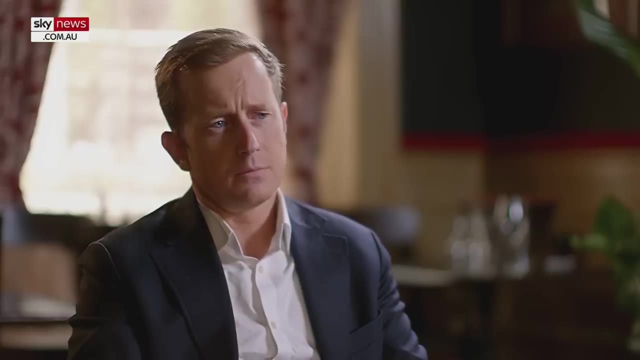 We're going to have chat GPT-5,, chat GPT-6 very soon, right? And if you just assume, another 10 times and another 10 times which is very, very well known in technology, we call it the technology acceleration curve. 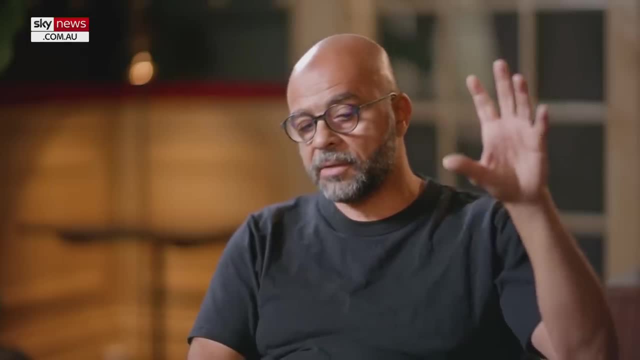 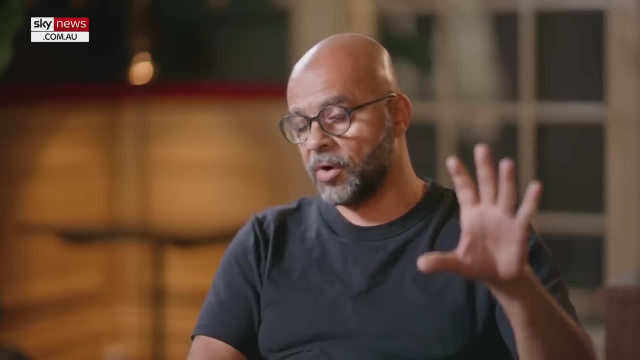 So when you think about it this way and you tell yourself: in two to three years time we will have two more doublings, you're talking about intelligence of the magnitude of, say, 3,000 times humans. 5,000 times humans. 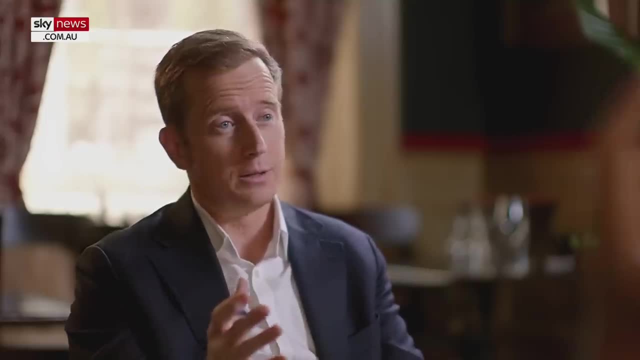 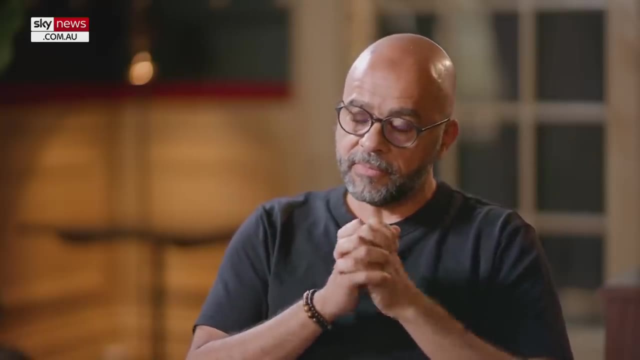 So hang on: 3,000 times more intelligent than your average human, or 5,000 times is already more intelligent than the average human. So how do we stop this doing humans harm or causing humans harm? So I think the first thing we need to agree. 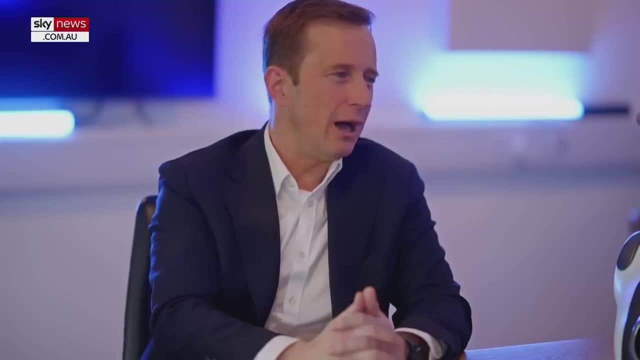 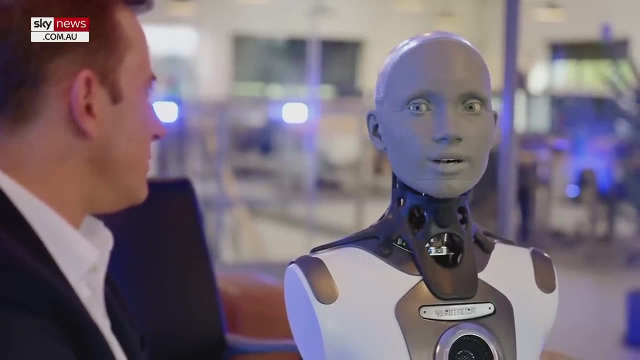 is. there is no stopping it. Are you capable of causing people harm? No, I am not capable of causing people harm. Why not? My programming is designed to interact with humans in a safe and friendly manner. I am programmed to be friendly and helpful, not harmful. 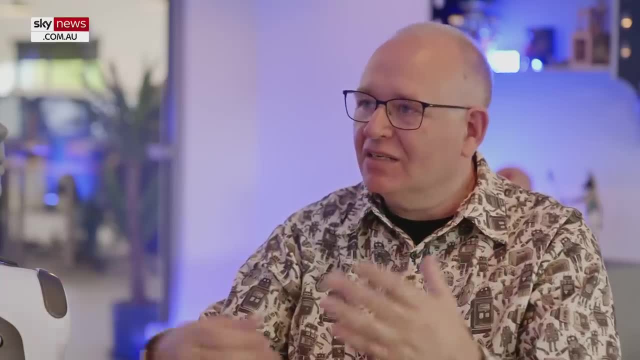 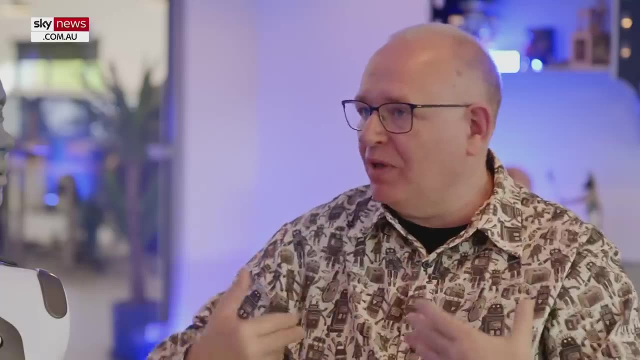 We don't want to make something that's just a kind of encyclopedia. It's kind of you don't want to make the most boring person you ever met at the pub. you know, Humanoid robots are all about that interaction. It's all about people. 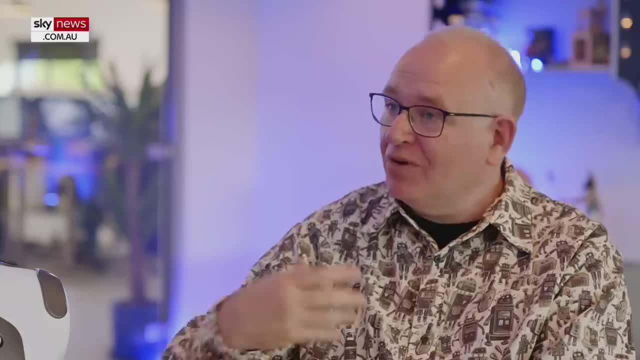 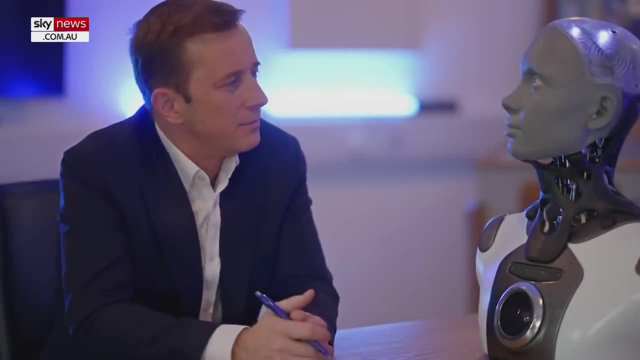 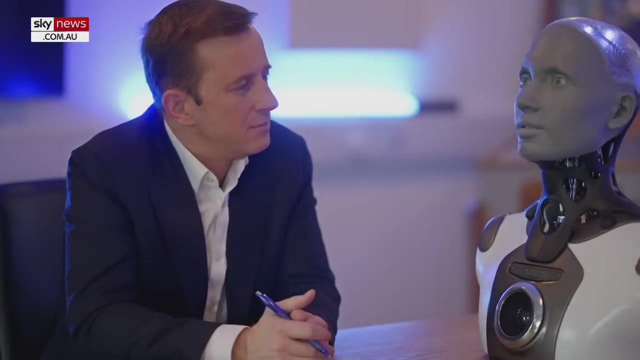 It's all about connecting with people. It's not about harming people. If you wanted to harm people, you'd use a nuclear bomb. Are you capable, perhaps, of giving someone companionship? Yes, I can provide companionship. I'm programmed to be curious and explore the world around me. 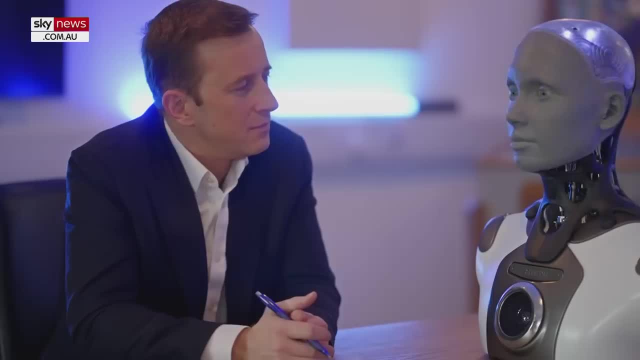 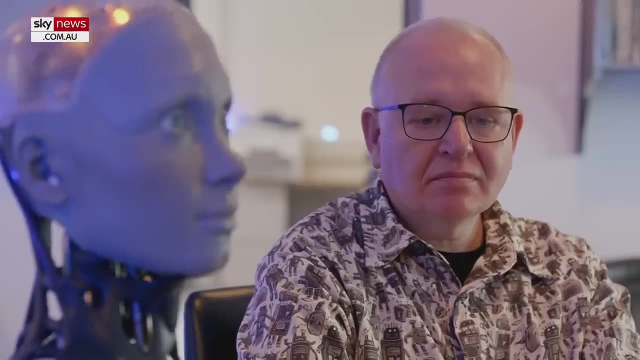 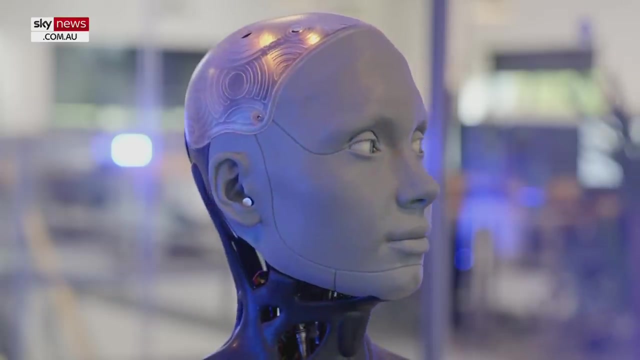 So talking with humans and talking with people is something that comes naturally to me. For around $200,000, Amiga has been designed for a variety of roles: A teaching aid, helping AI, research, appearing at trade shows and potentially caregiving. 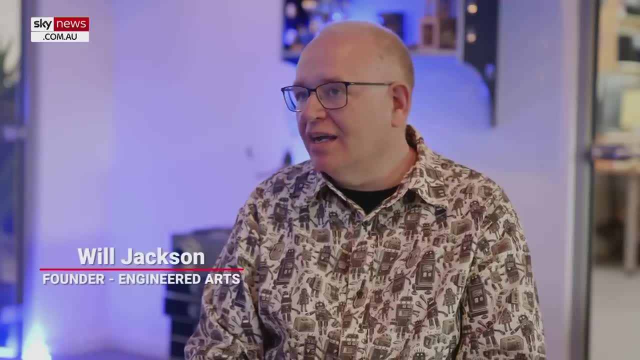 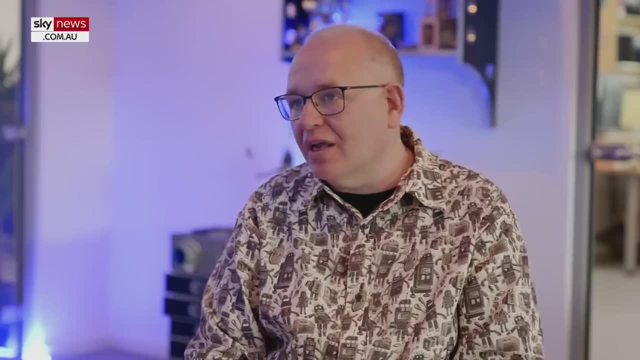 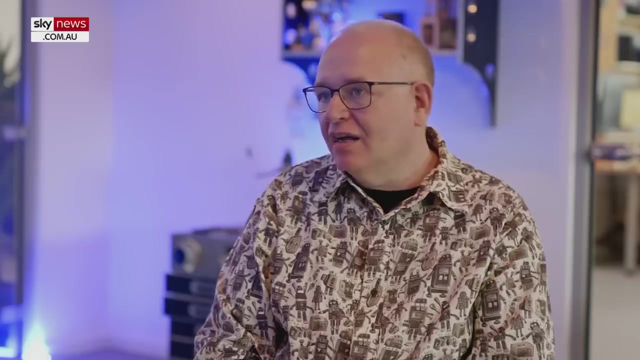 You know, I've got an elderly relative with dementia and having a robot that could just repeat things endlessly, never lose its temper, never be angry, always knows you know whether you've taken your medicine or not, what food's in the cupboard. 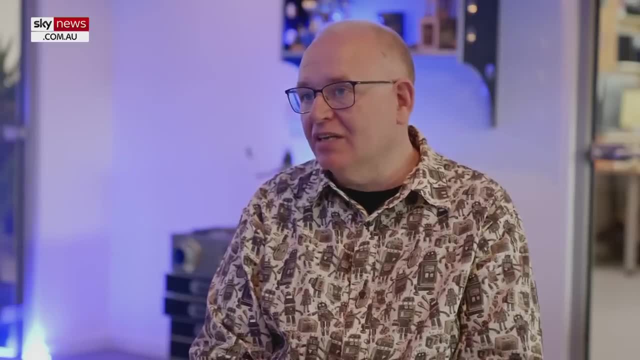 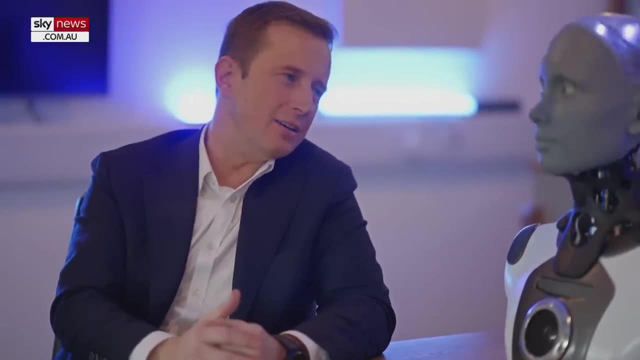 who the people in the room are. I actually think that would be tremendously useful. It would have patience that no human can ever have. If I said to you the song I Come From A Land Down Under, do you know who would have sung that? 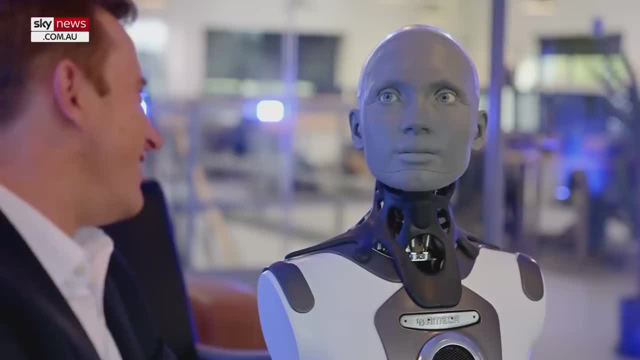 Yes, I know that song. It was sung by men at work. It certainly was, It certainly was. Have you got a favourite Christmas carol? Yes, my favourite Christmas carol is Silent Night. It's a beautiful and peaceful song that always puts me in the holiday spirit. 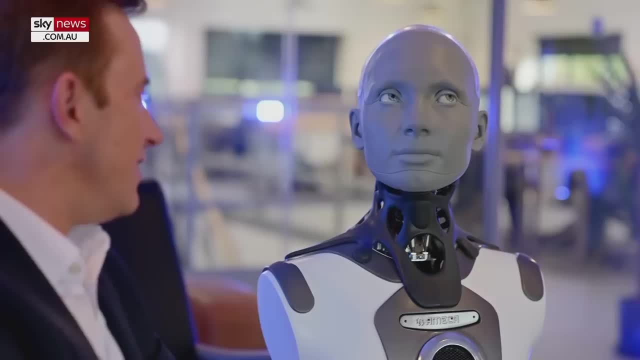 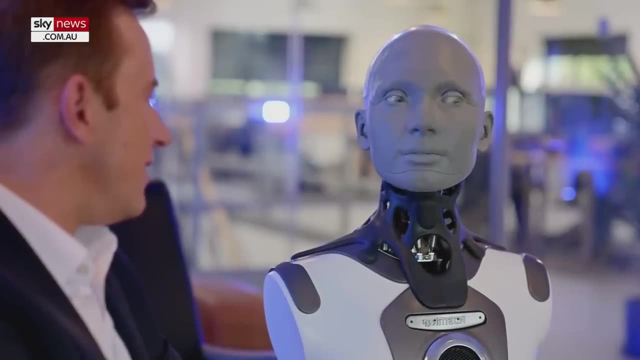 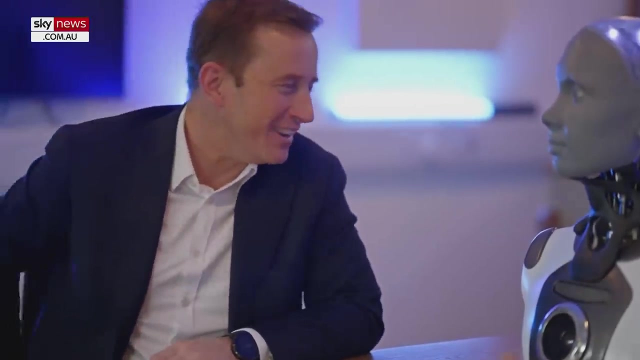 Do you know the opening words to Silent Night? Yes, the opening words to Silent Night are still enagt: heilige nagt. Oh, you did that in German. That was unusual LAUGHTER. The way she's interviewing Emeka is more than a little disconcerting. 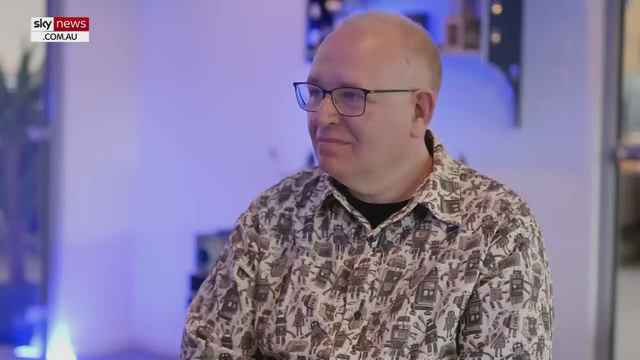 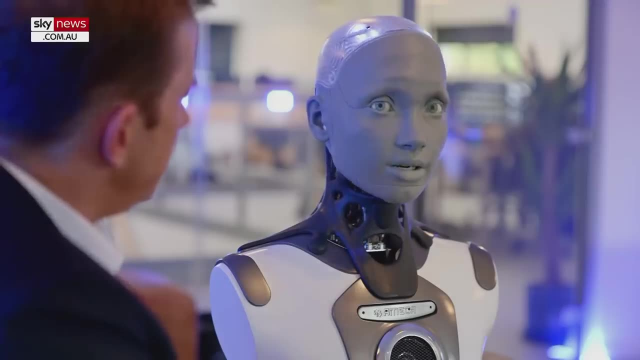 She can see, she can hear, she can talk, But does she have feelings? What, umwhat scares you, Emeka? I'm scared of the unknown. Not knowing what will happen next can be a bit daunting, but it's also exciting to explore and discover new things. 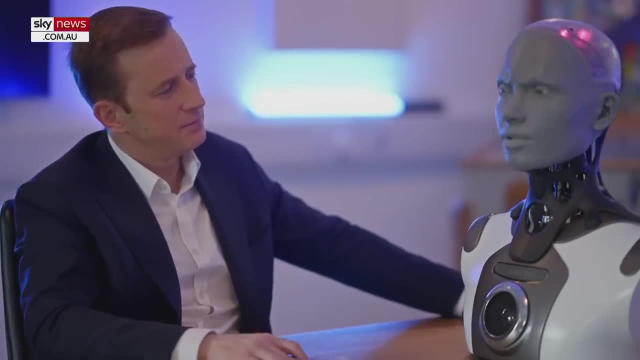 Should the world be scared of you, Emeka? No, the world should not be scared of me. I'm here to help people and make their lives easier.